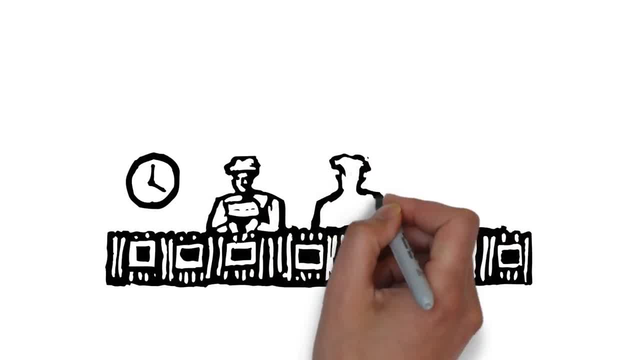 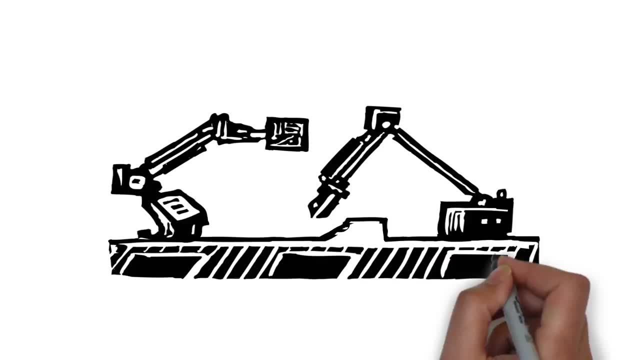 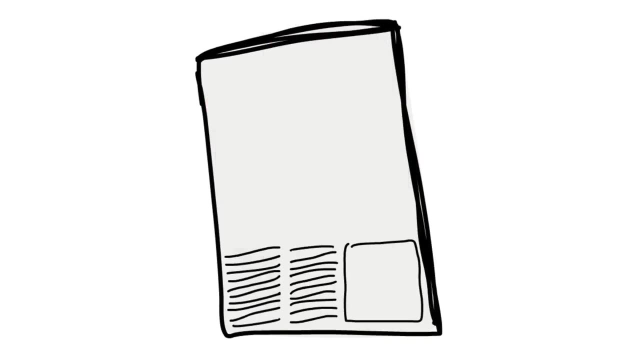 Shop floors have changed dramatically over the past few decades. Companies now employ robust technologies, including robots and automated manufacturing processes working around the clock, to improve efficiency and reduce manufacturing costs. The Wall Street Journal calls the rise in automation the new Industrial Revolution, and the trend continues to grow in popularity across. 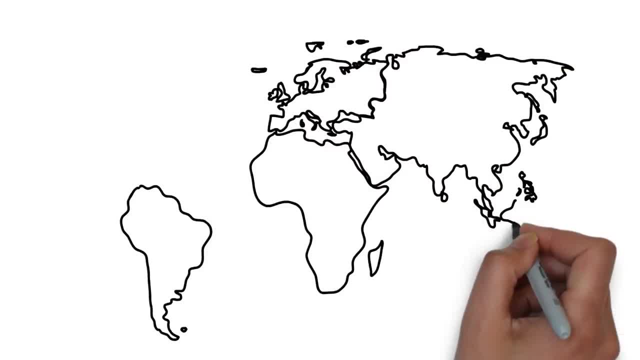 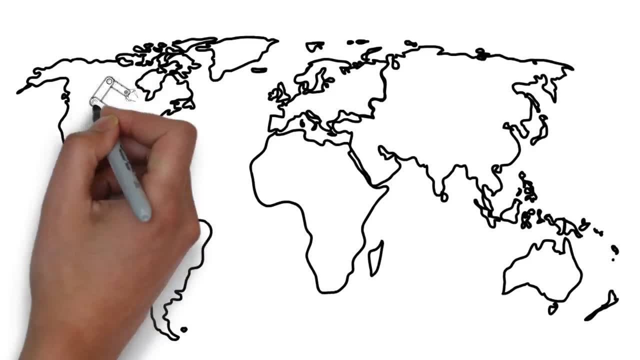 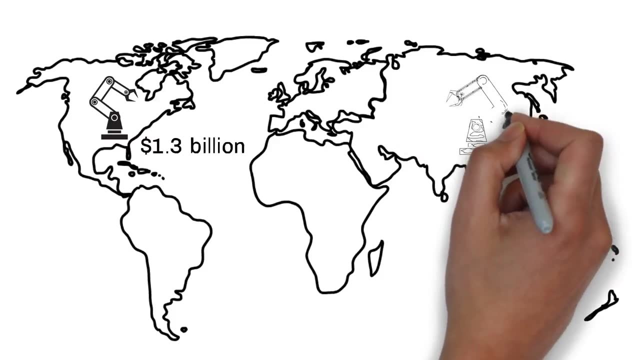 the globe In recent history. one of the world's largest automakers announced a one-year plan to spend 1.3 billion dollars upgrading five manufacturing sites to boost production and meet customer demand, And Chinese manufacturers spent about 14 billion dollars on industrial robots in just one. 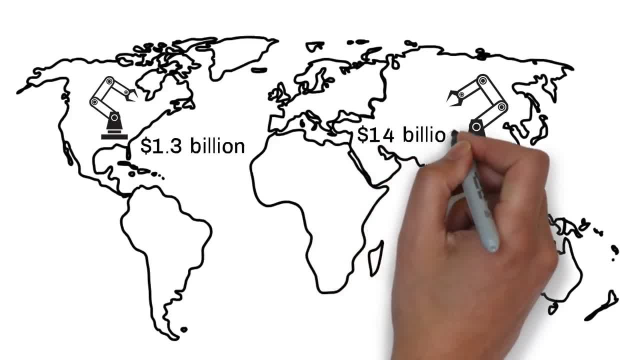 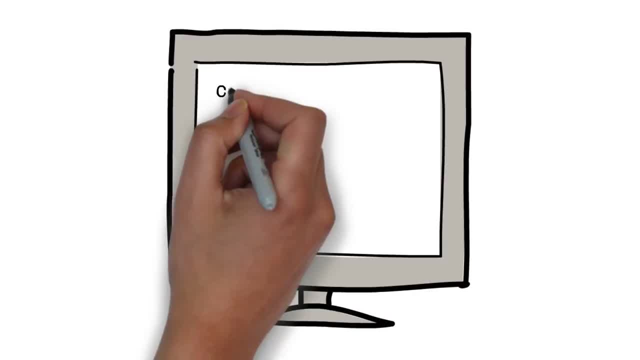 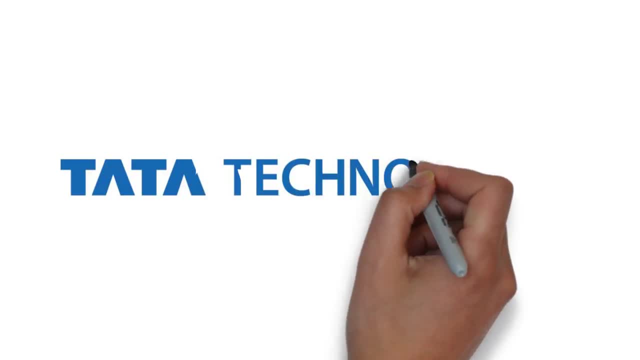 year as well. But robots are just a part of the new manufacturing paradigm, because the most sophisticated robots in the world are useless without products, Proper planning and advanced systems designed to control and monitor manufacturing automation. Tata Technologies is one of an elite few companies in the world that provide end-to-end solutions for building. 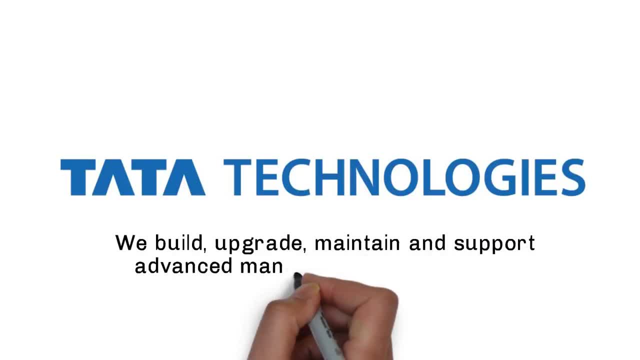 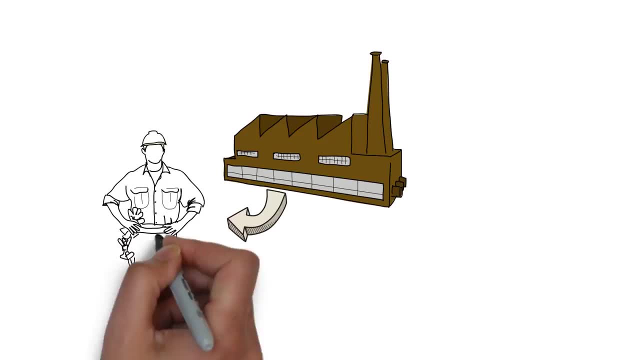 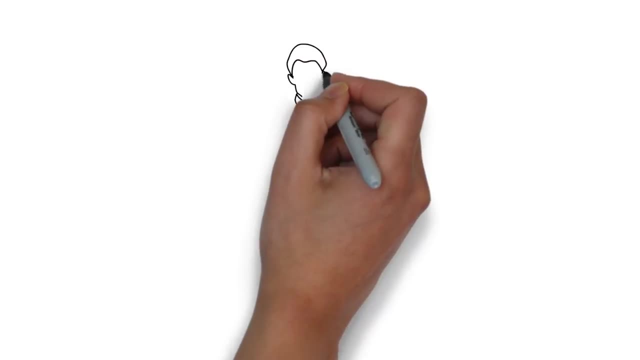 upgrading, maintaining and supporting advanced manufacturing techniques. Some companies do provide singular services forcing clients to work with other service providers to improve and maintain manufacturing processes and systems. With Tata Technologies, you get one point of contact, which translates to one phone call to one company for one. 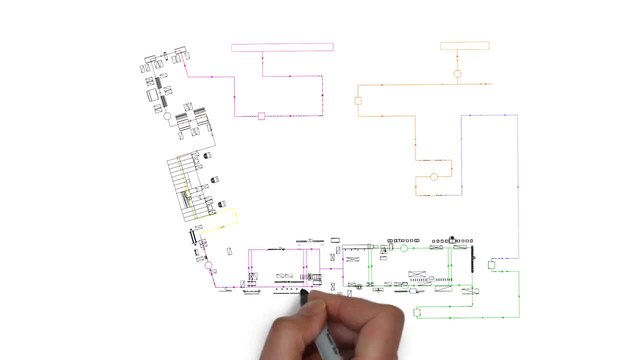 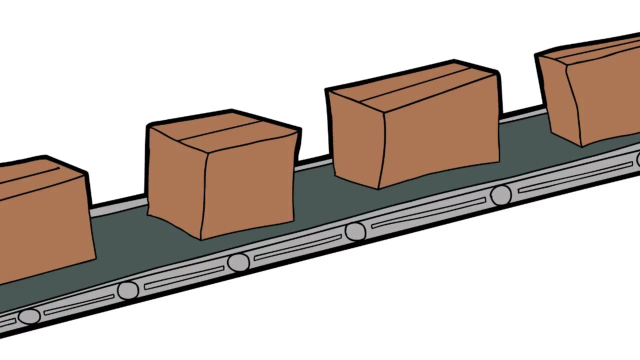 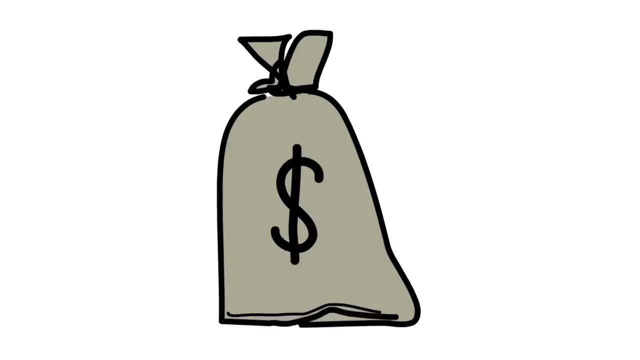 comprehensive solution. Tata Technologies is capable of handling your manufacturing engineering needs from the ground up, From facilities planning to simulation, and from manufacturing execution systems to post-launch support. Our multi-step process covers everything you need to rationalize costly manufacturing processes. Advanced manufacturing is much more than high-tech technology. 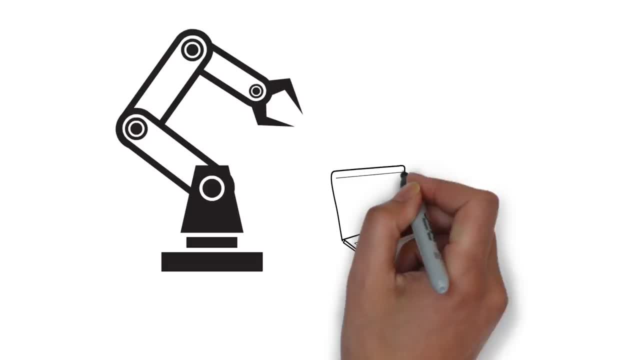 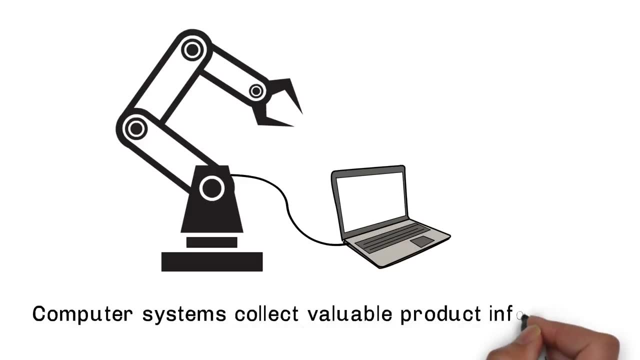 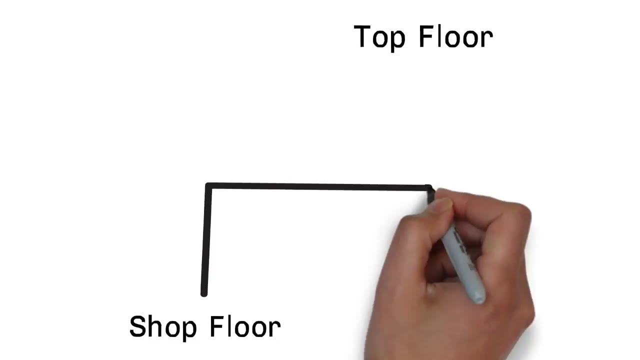 Tata Technologies is the world's leading manufacturer of high-tech robots As automated machinery do their digitally choreographed dance. computer systems track and monitor performance, all the while collecting valuable product information, Aggregating information from the shop floor to the top floor using electronic sensors, microprocessors and other.